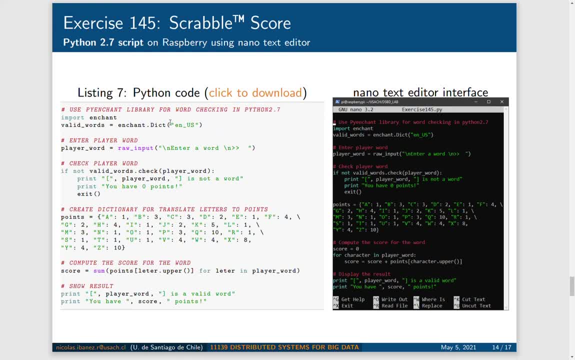 So I will tell you how I solved this problem. First I import the enchant library with the command import, then I create an object validWords for English spell checking. then I store the used word as a string with the command row input in the variable playerWord. 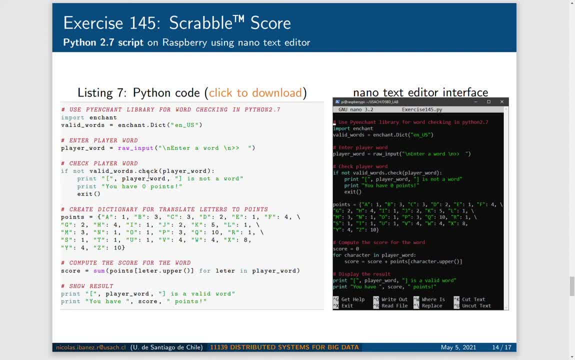 Using the check method to the validWords object, I can check if the playerWord parameter is spelled correctly. So if this conditional sentence is false, the program shows the player that his word is invalid. therefore his score is 0. then the program closes. In case the word is valid, a dictionary is created. 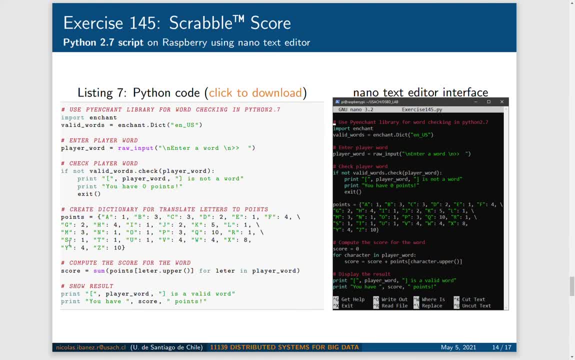 where the keys are equal to the letters and the values are equal to the points of the letters. The score is calculated adding all the points of the letters extracted from the available playerWord converted to uppercase using a list comprehension as a parameter of the sum command. 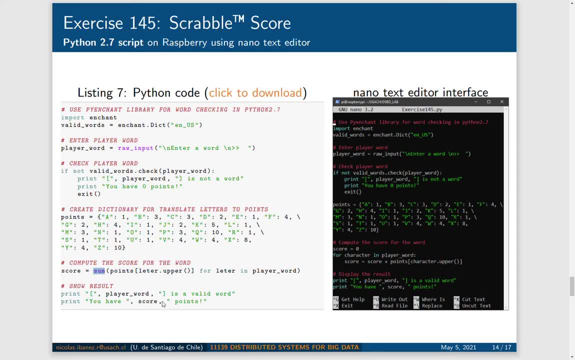 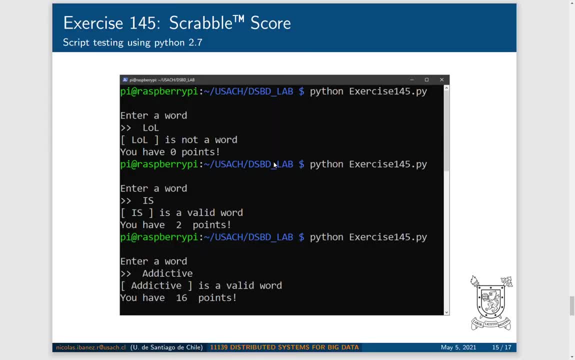 And finally the program displays the playerWord score. Ok, We can see in this script that the program works. Thank you for your attention. 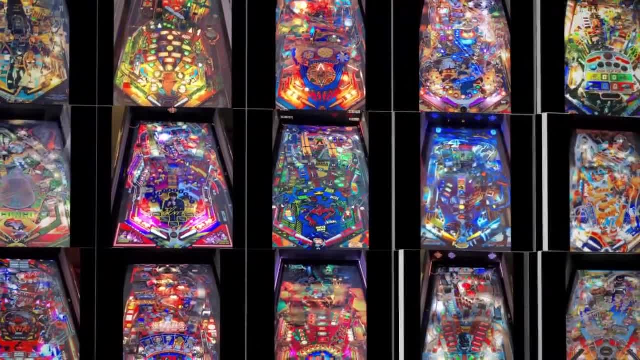 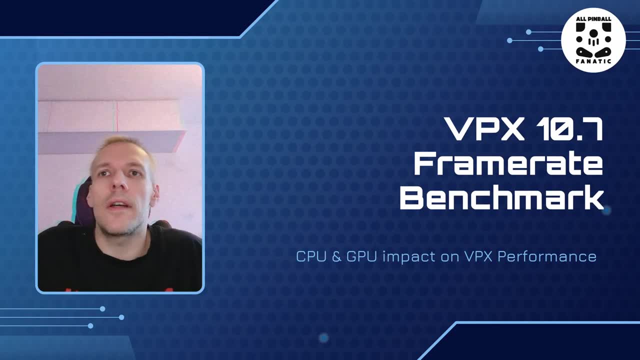 Hi Luke here, all pinball fanatic, I would like to present you today my findings about frame-per-second performance in Visual Pinball X and the impact of the core PC components on it: the processor and the graphics card. I think my findings can be interesting to some of you thinking of changing 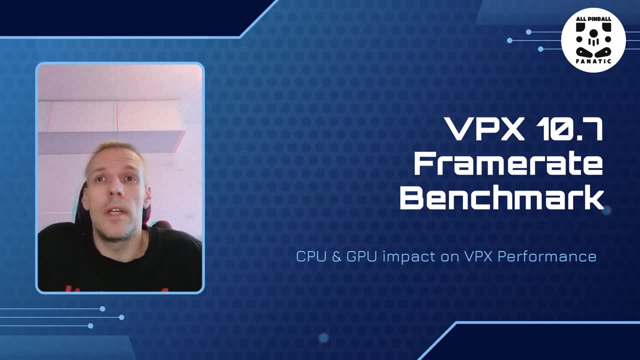 the components of their Visual Pinball cabinets. For some time I've been struggling to get 100% fluent performance in VPX to achieve what I think is the most important in Virtual Pinball: stutter-free gameplay with no hiccups at all. What drives me crazy is the moment when ball goes.